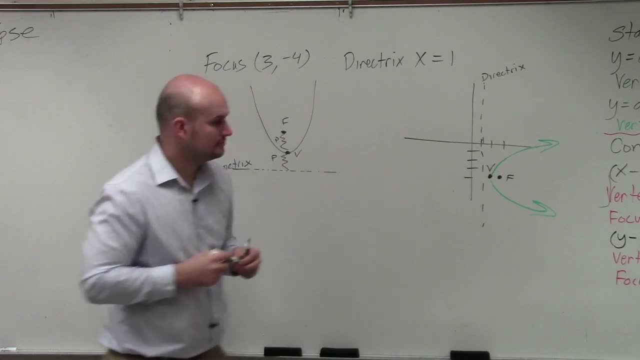 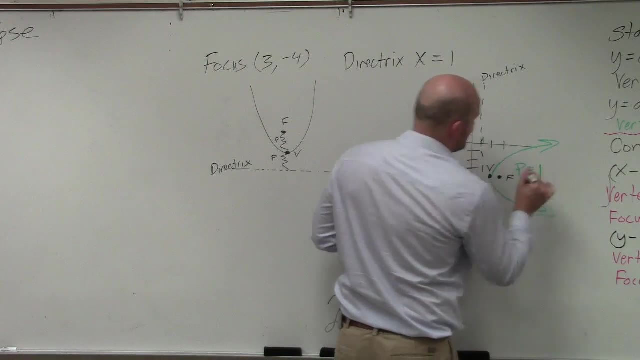 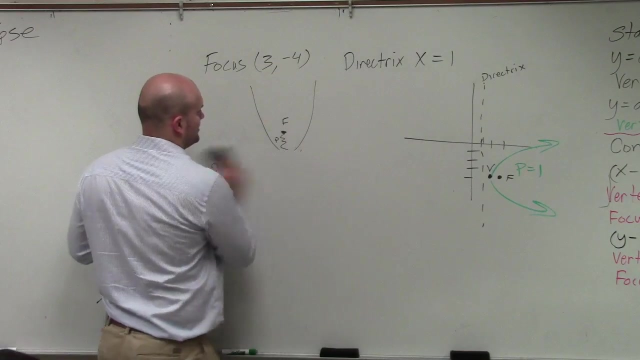 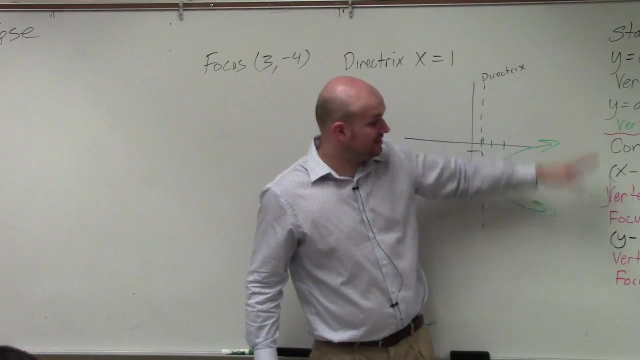 Right. And then we can also identify that the distance from the vertex to the focus, P, is equal to 1, which is positive. That's very important. It's going to the right, All right. So when you type in your phone, what I'd like you to do, then, is identify which formula we're going to be using. Here x squared, That's like what you've previously studied. Here y is squared, So that means it's going to be opening right or left, So that's the formula I'm going to use. 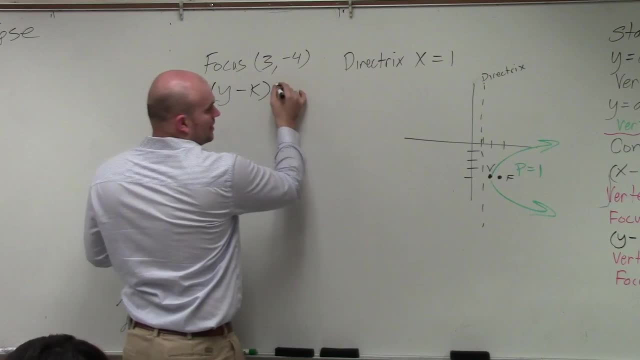 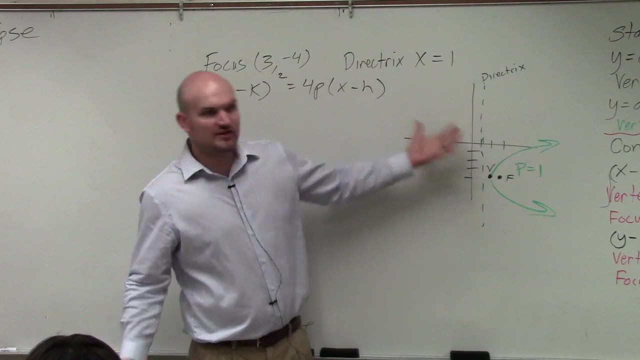 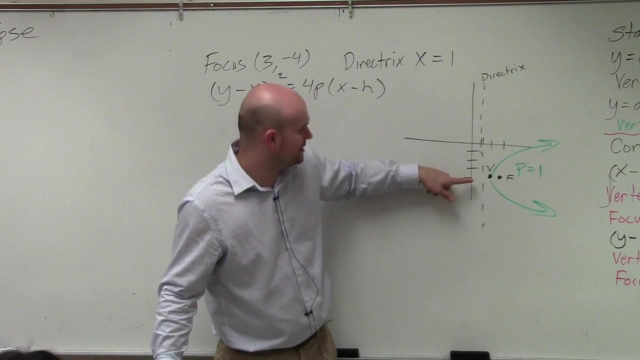 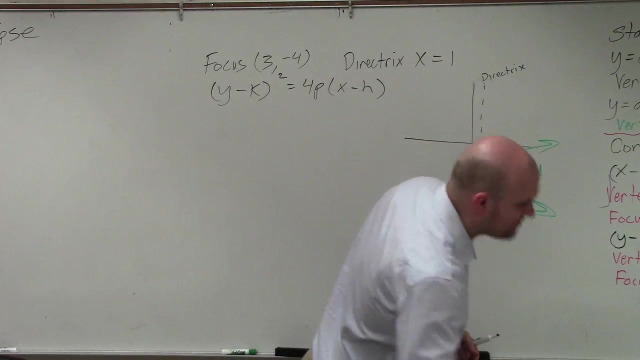 So I just type in: y minus k squared equals 4p times x minus h. Since I plotted the points, can you guys just kind of figure out from my makeshift graph of what the coordinates are for the vertex? Yeah, it's just going over 2, down 1, 2, 3.. Is that supposed to go down 3?? What was it? 4.. Okay, Down 1,, 2,, 3, 4.. And the other thing that's important is: I know that my vertex 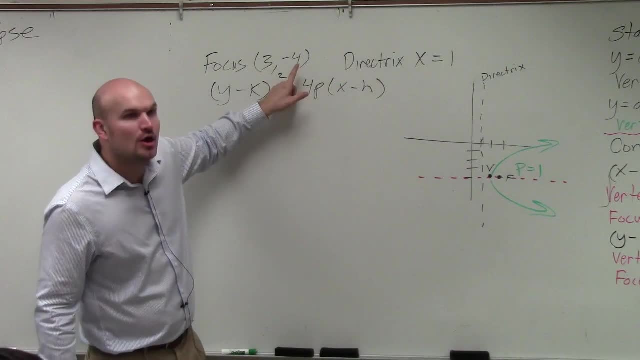 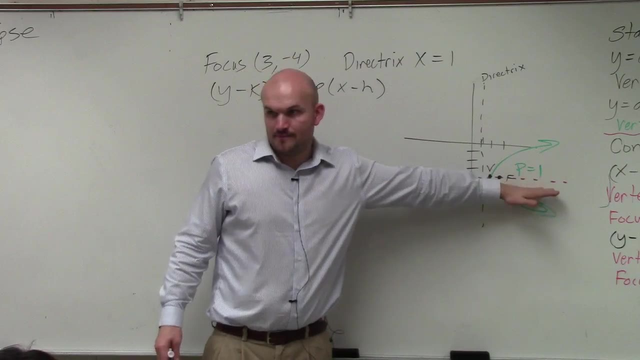 has to have the same y coordinate as my focus. Why? Because the vertex and the focus always are on the axis of symmetry together. Right, So they have to share the same y coordinate because they always are on the same axis of symmetry. Yes, 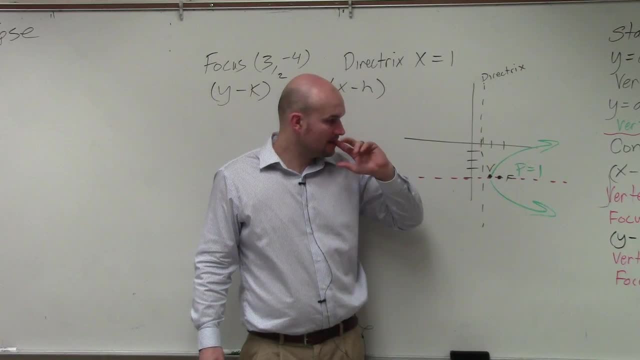 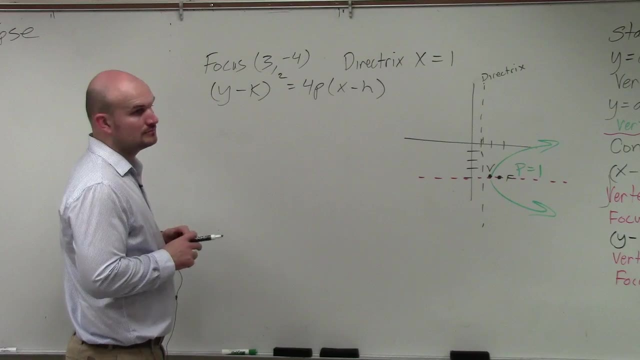 Okay. now when it says y minus k, squared so say we have, say our k is equal to: oh, that's just for the vertex, not the vertex right, Like h and k is the vertex right Huh. 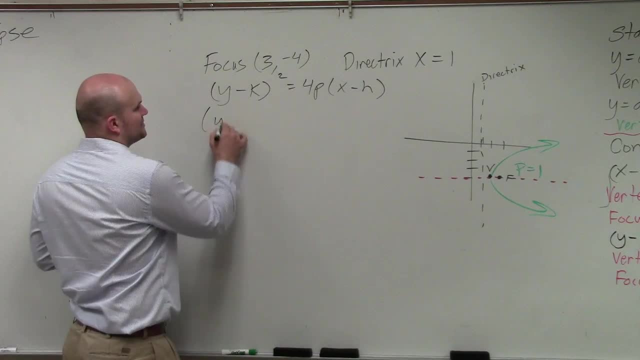 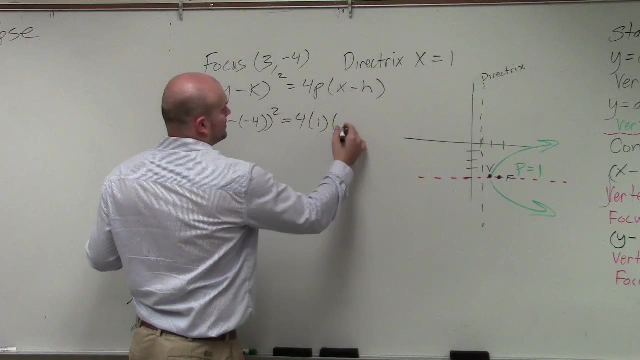 H and k is the vertex, okay, and then y. if you think So, we just do y minus negative 4 squared. yep, that will go. I'm just writing it in there: times 1 times x minus 3.. 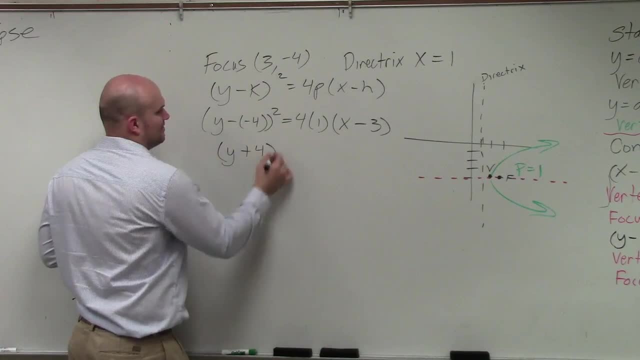 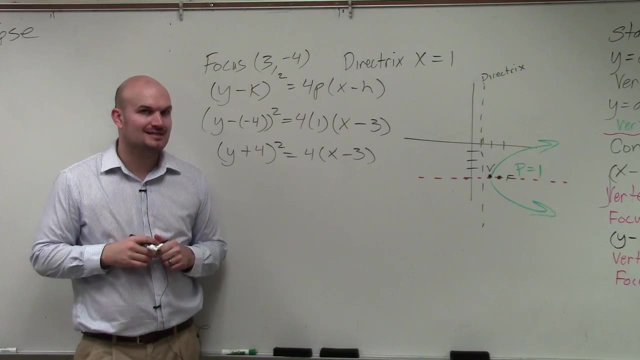 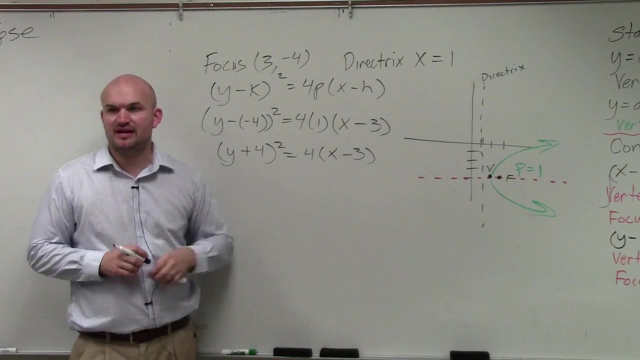 So Would that be a double or a negative? That's why we get the positive. And there's our equation: Done, Sleep, Just like that. perfect, Because then it's really easy to find p, right? You know that 4p is equal to 4, p equals 1, right? So, yeah, we like to factor it off.